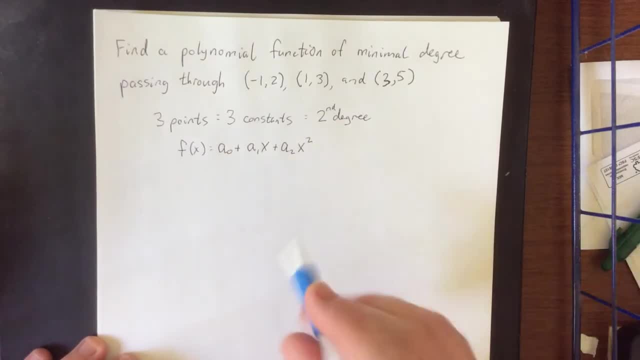 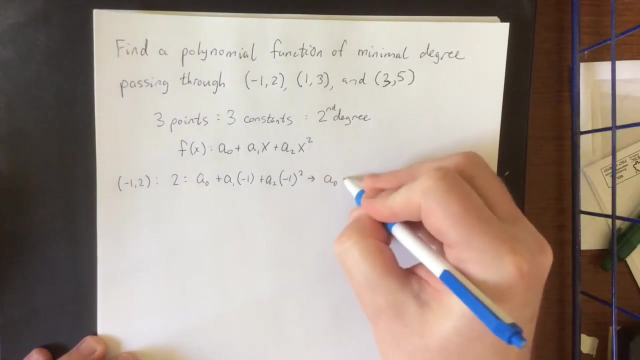 for these unknown constants, a naught, a1, and a2.. So the interpretation that we can give to negative 1, 2 is that the y value will be 2 when the x value is negative 1.. Now, putting this into more of a standard form, we'll call this a naught minus a1 plus a2 is equal. 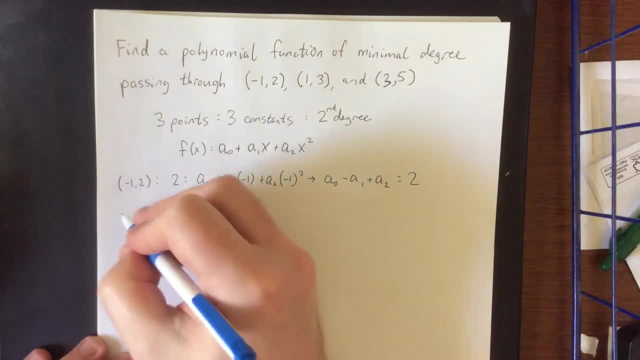 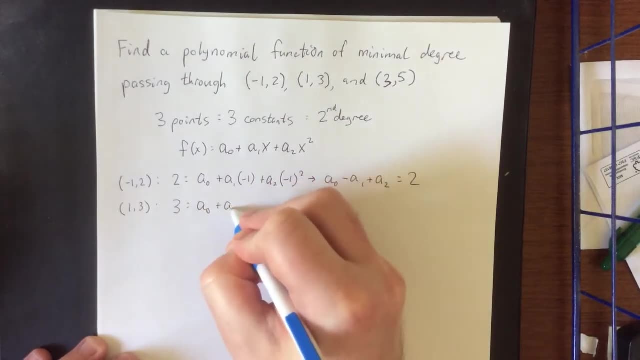 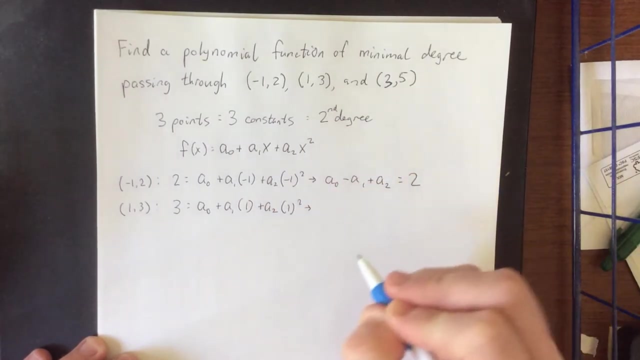 to 2.. That'll be the first row in our matrix. once we set this up For similar sort of concept, y value will be 3 when the x value is 1.. And again, rewriting this slightly: A naught plus a1 plus a2.. That's going to be equal to 3.. 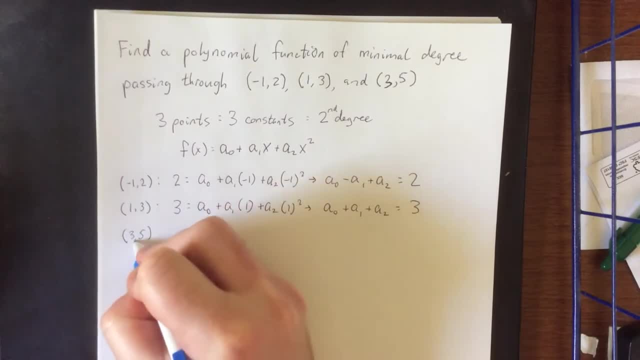 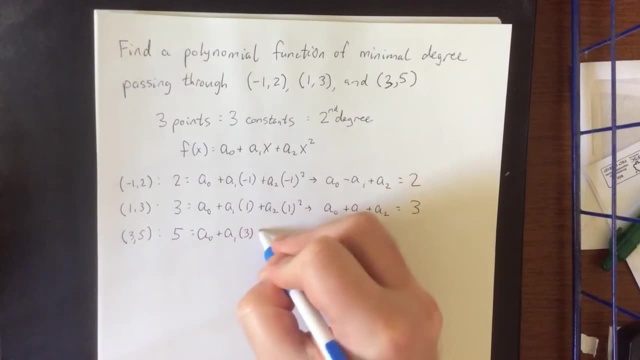 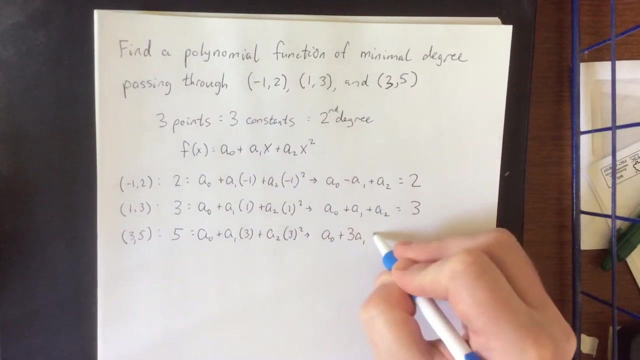 And then for the last one, that's 3, 5 means that the y value is going to be 5 when we plug in, x is equal to 3.. so a naught plus 3 a1 plus 9 a2, that's going to be equal to 5.. So what results is a system of three equations with three variables. 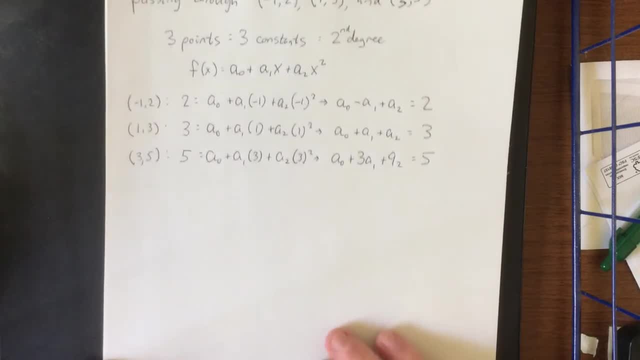 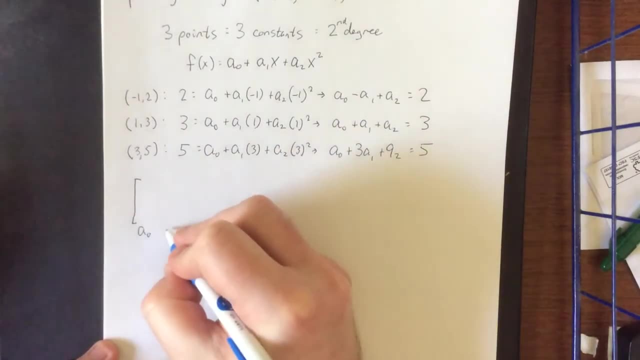 that we're going to be solving for We'll set that up using a 3 by 4 augmented matrix. The first column will represent the constant a naught, second one will be a1,, third one will be a2, and then, to the right of that, we'll have what it's equal to. So interpretation of the first. 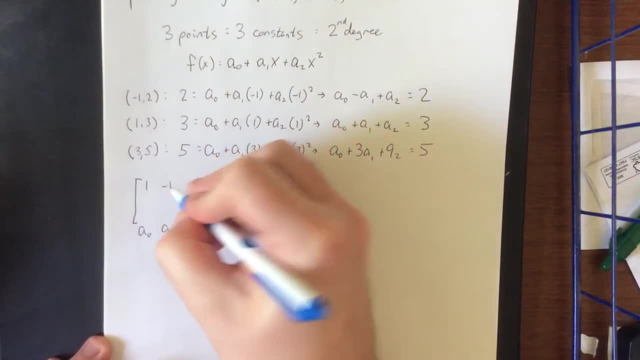 equation, as the first row coefficients are 1, negative 1, 1, 2.. Second row coefficients are 1, 1, 1, and it's equal to 3, and for the third equation this would be 1,, 3,, 9, and it's equal to 5.. 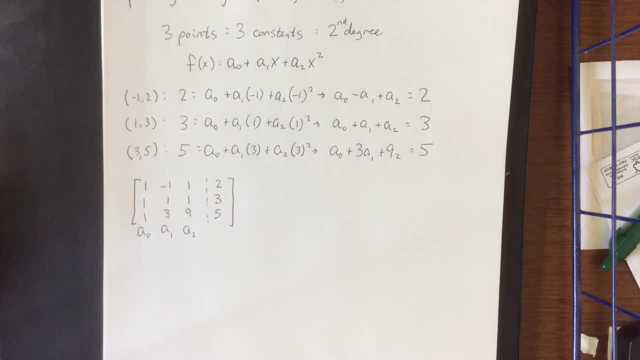 Now what we're going to try to do here is put this into reduced row echelon form. So the very first thing I'm going to do is notice that I already have my lead 1 in the position where I want it, which is the 1, 1 entry. 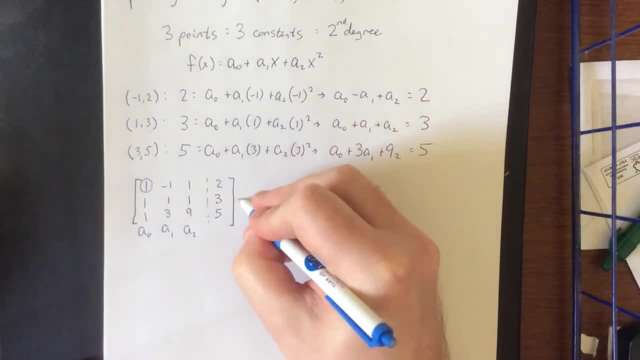 We're going to use this 1, 1 entry to zero out the two entries that are below it. We can do so by taking negative 1 times row 1, adding it to row 2, and having that become the new row 2, and do the same thing to row 3.. Negative 1 times the first row. 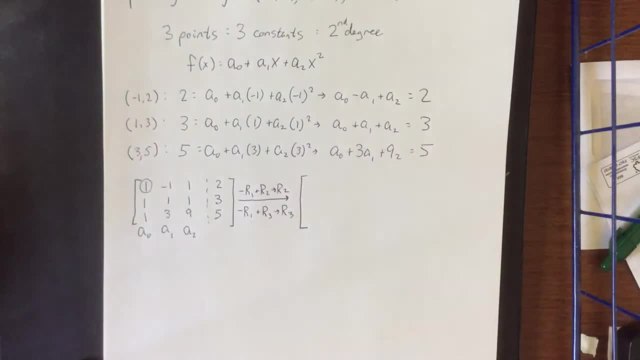 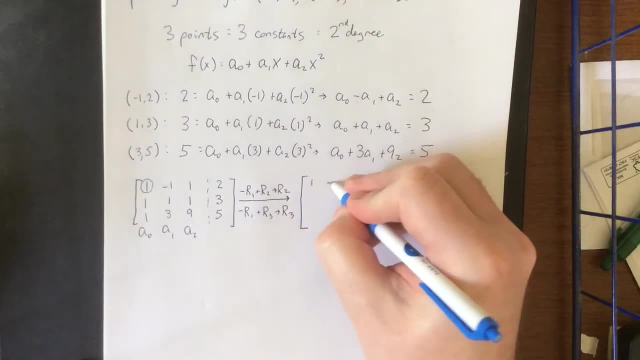 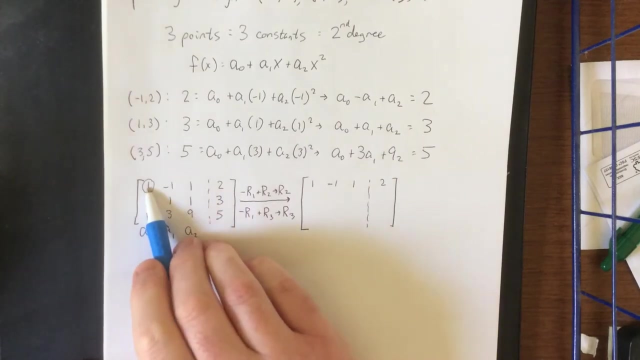 add to the third row, that'll become the new third row. Negative 1 times 1,. oh sorry, I'm going to recopy the first row, since that is not changing. We'll take negative 1 times 1,. add to 1, we'll get 0.. 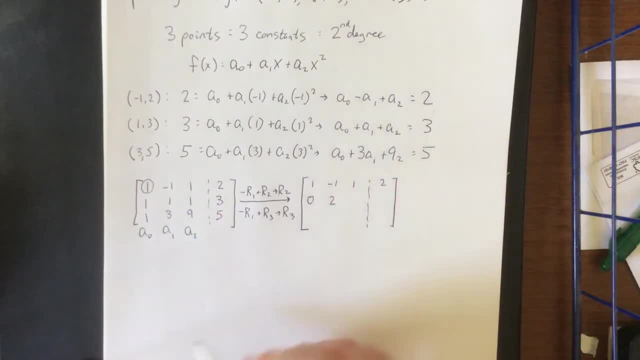 Negative 1 times negative: 1, add to 1, we'll get 2,. and negative 1 times 1, add to 1, we'll get 0. And that right, there is an absolute gift. We're also doing negative 1 times 2, add to 3,. 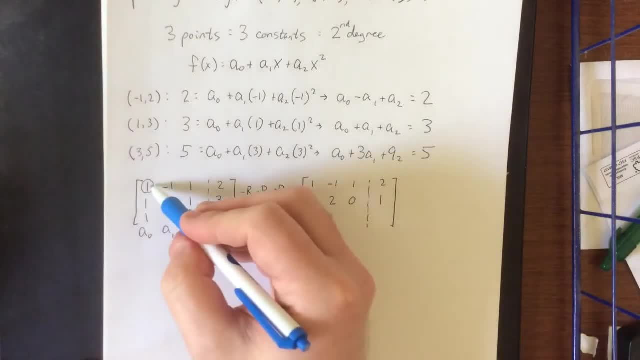 and that's how we get this 1 here. So we're going to take: negative 1 times 1, add to 1, we'll get 2, and negative 1 times negative 1, add to 3, we'll get 4.. Negative 1 times 1, add to 9, we'll get 8.. Negative 1 times 2,. 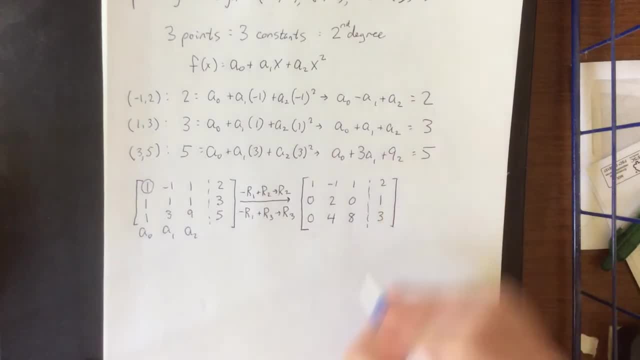 add to 5, we will get 3.. Now that we've zeroed out all of the other entries in the first column, we're going to sort of ignore the first column and ignore the first row and just worry about the second and third rows and treating this as its own little thing. So we're going to do that. 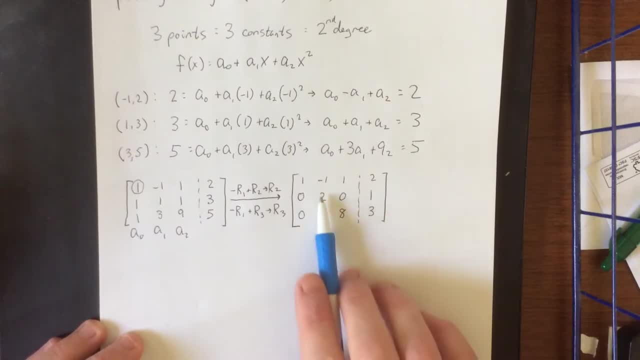 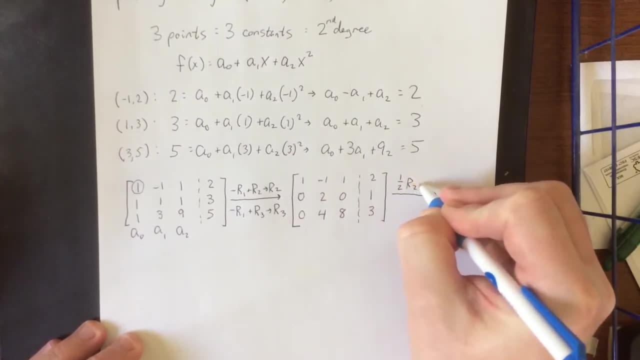 We're going to take a simple 2 by 3 augmented matrix. First thing I want is a 1 in the 2,2 entry. I'm going to accomplish this by simply taking half of row 2 and calling that the new row 2.. 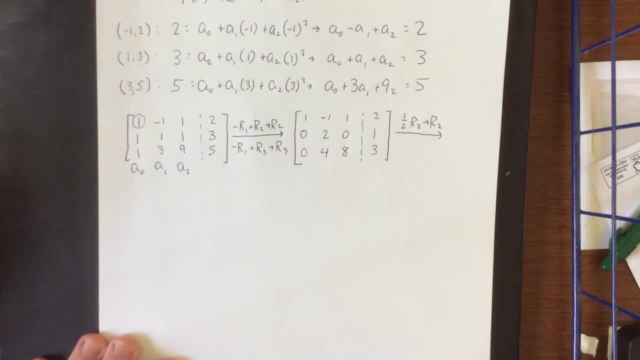 It will introduce a fraction. I'm not happy about that, but I'm pretty sure the fractions are going to be unavoidable on this one, so we might as well get used to it. First row remains the same: 1, negative 1, 1, augmented with 2.. The second row: we're going to take a 2 by 3, and call that the new row 2.. The second row: we're going to take a 2 by 3, augmented with 2.. The second row: we're going to take a 2 by 3, augmented with 2.. 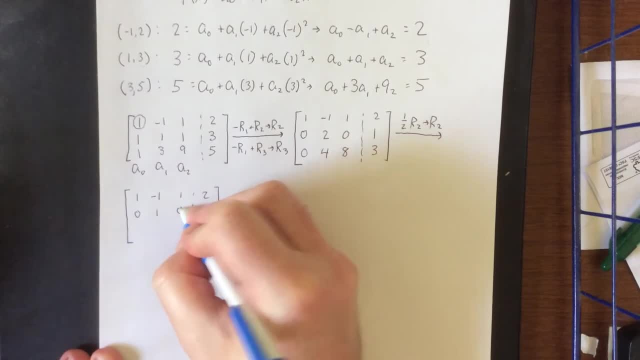 The second row: we're going to take a 2 by 3, augmented with 2.. The second row: we're going to take a 2 by 3, sebagai 1 in the row 2 and thanked for that. The third row remains the same. We only have half of the entries. 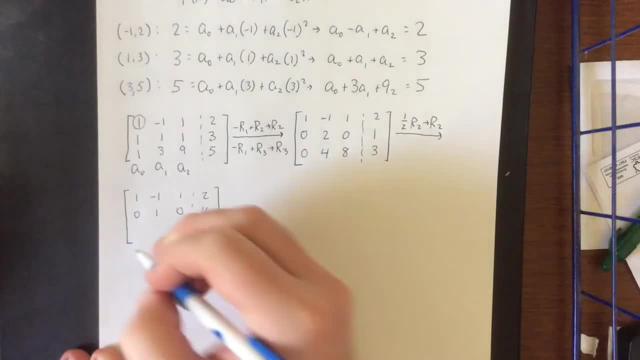 That provides us 0,, 1,, 0,, 1.5 for the four entries of that row. The third row remains unchanged. Now that we have our lead one in the entry, next thing to do is going to be to zero out the entries above and below it. 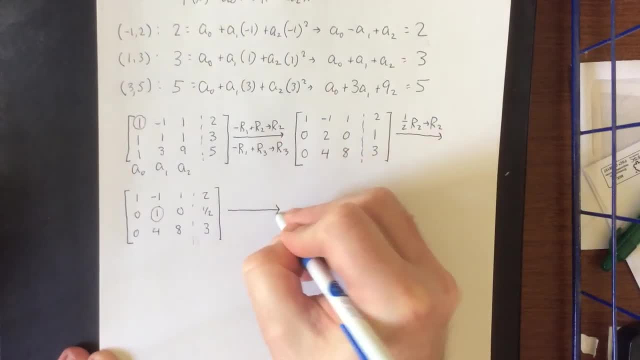 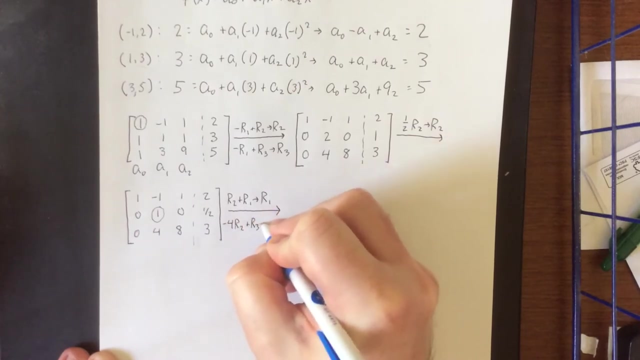 So, zeroing out what is above and below it, we get reduced row echelon form. we're going to take row 2 added to row 1 to become the new row 1.. We'll also take negative 4 times row 2, add to row 3, that'll become the new row 3.. 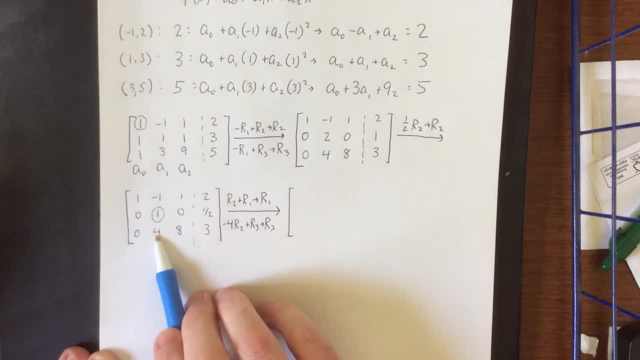 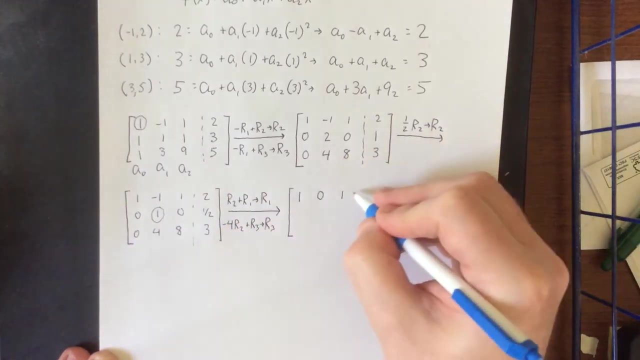 That'll use this lead 1 to 0 out the entries above and below it. So, adding these together, 0 plus 1 will be 1,, 1 plus negative 1 will be 0,, 0 plus 1 will be 1, and 1 half plus 2 will be 5 halves. 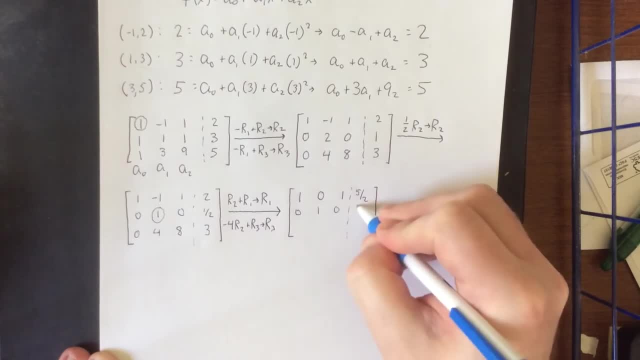 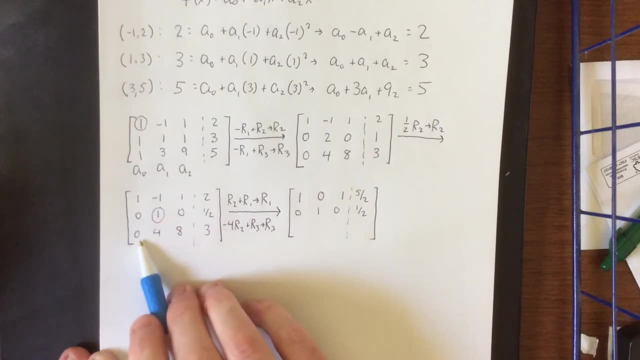 Second row remains unchanged, And taking negative 4 times the second row and adding to the third row, negative 4 times 0, add to 0, will remain 0. That's why we like those zeros there. Negative 4 multiplied by 1, add to 4, we'll get the 0 that we desired, and 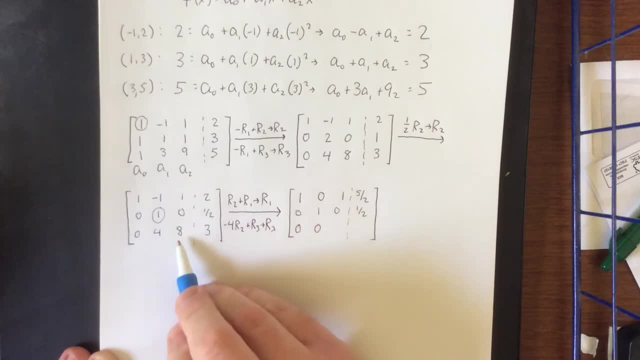 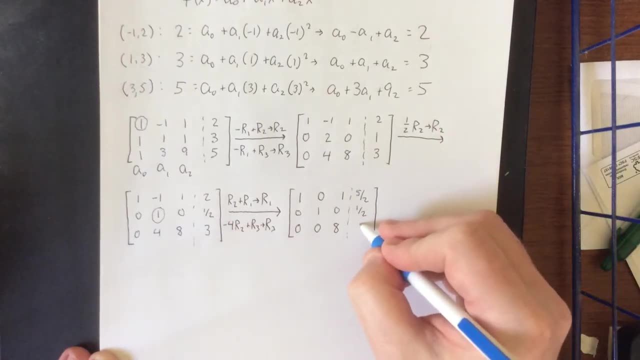 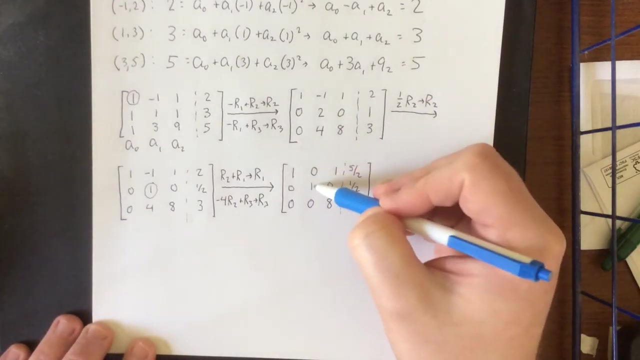 then negative 4 multiplied by 0, add to 8, we'll get 8.. Negative 4 times 1: half is negative. 2, add to 3, we'll get 1.. Now that we have lead ones in the first and second row, we ignore the first and second row and focus on the third row. 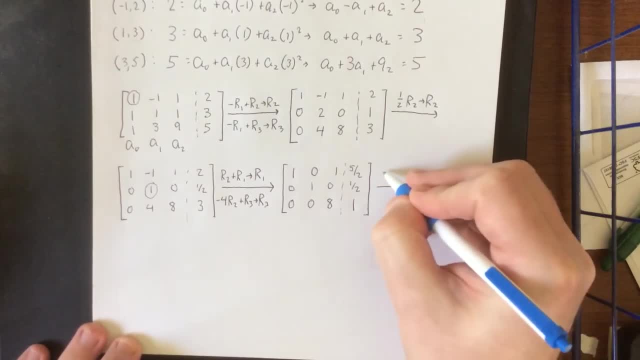 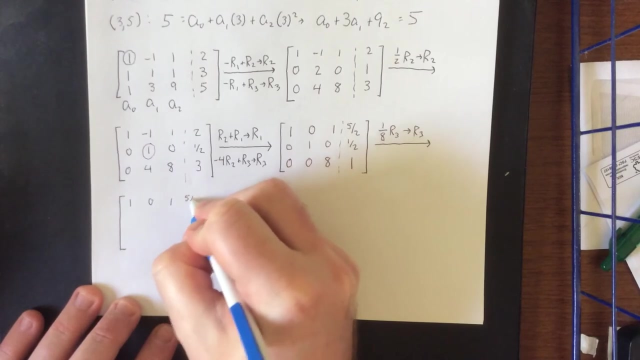 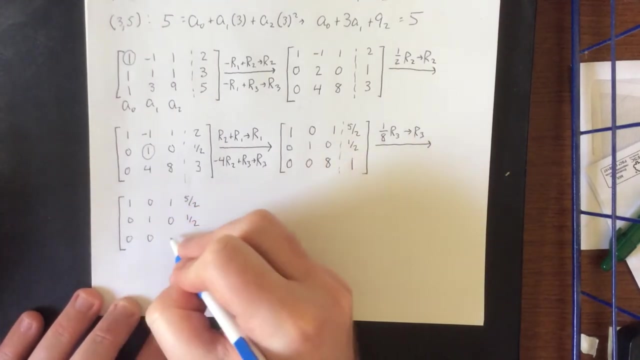 To get a lead one down there, we'll simply take 1 eighth times row 3, and that'll become the new row 3.. So first and second rows will remain the same: 1, 0, 1, 5 halves 0, 1, 0, 1 half 0, 0, 1 will be 1 eighth. 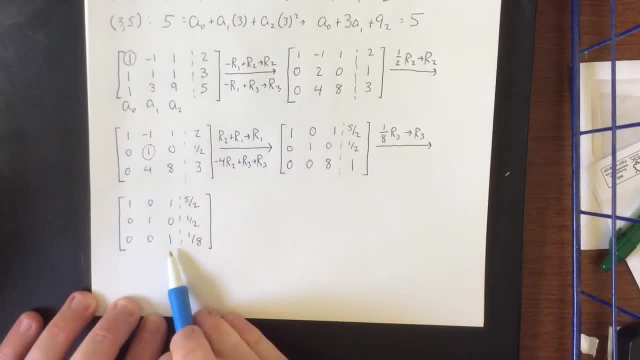 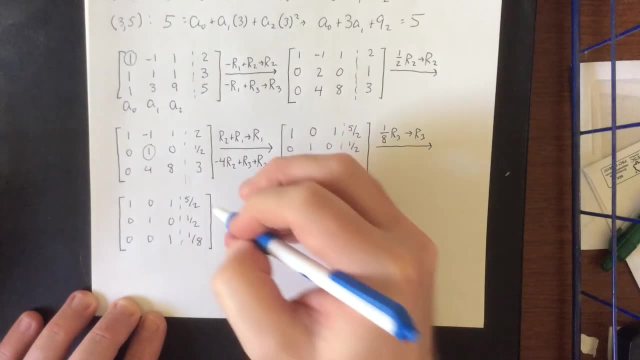 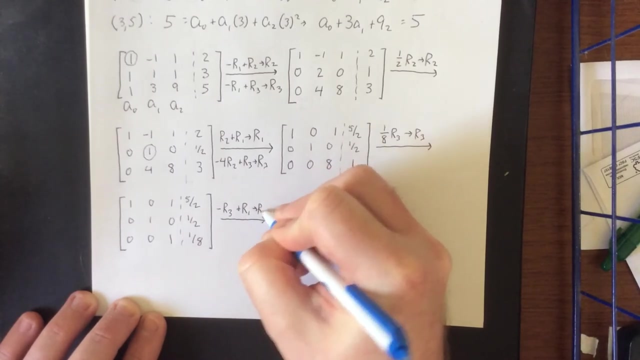 So we now have numerical answers For both a 1 as well as a 2, let's finish this off by getting a 0 in the 1, 3 entry. We'll do that by taking negative 1 times row 3, add it to row 1, that'll become the new row 1.. 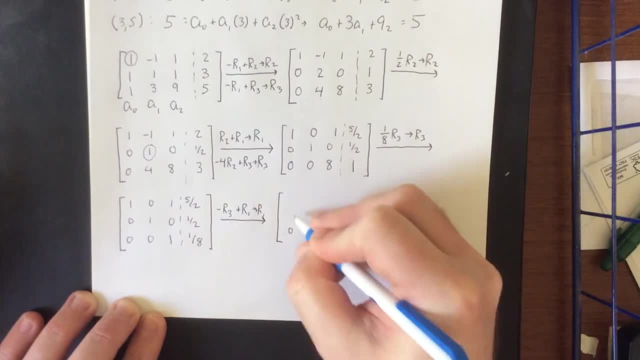 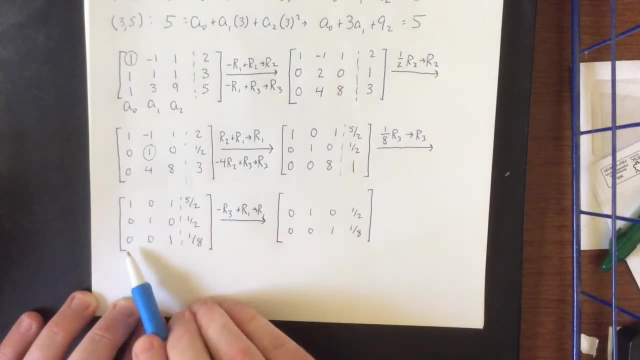 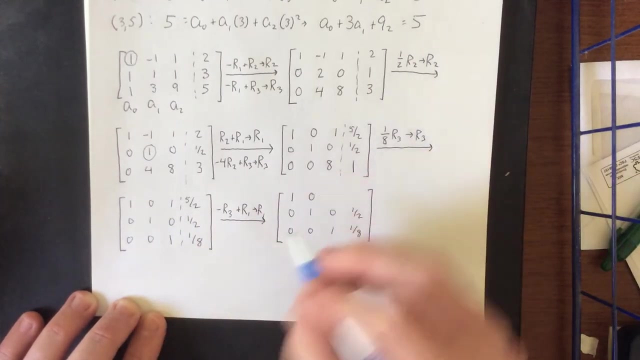 So third row remains the same, second row remains the same. and then: negative 1 times 0, add to 1, we'll be 1,. negative 1 times 0, add to 0, we'll be 0,. negative 1 times 1, add to 1, that'll be 0,.